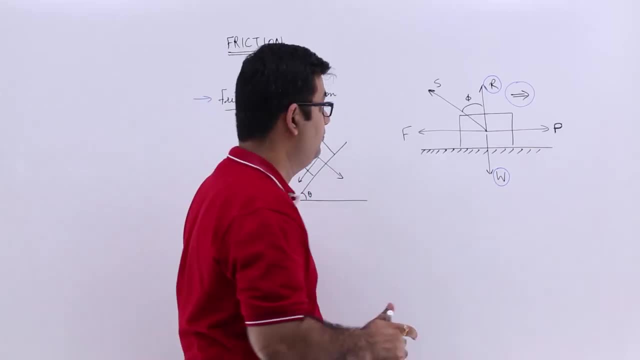 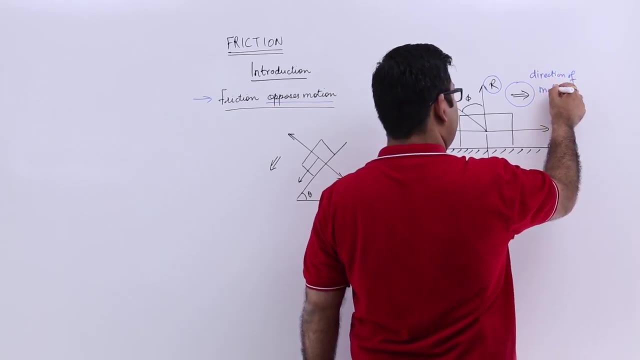 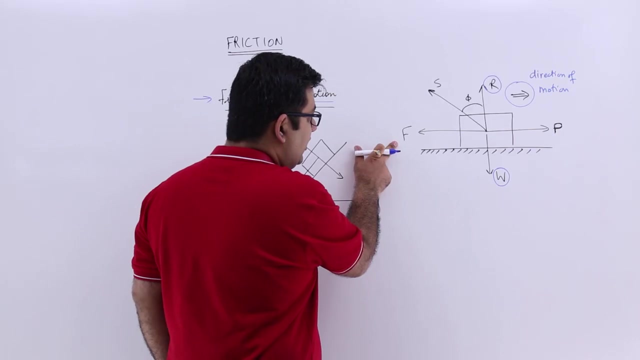 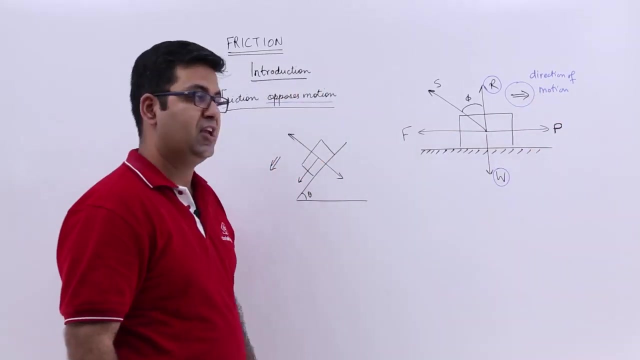 arrow denotes the direction of motion. Okay, so this is the direction of motion. Now, as I told you that friction is a force which opposes motion, So frictional force, here denoted by letter F, is in the opposite direction to that motion. So this is F which. 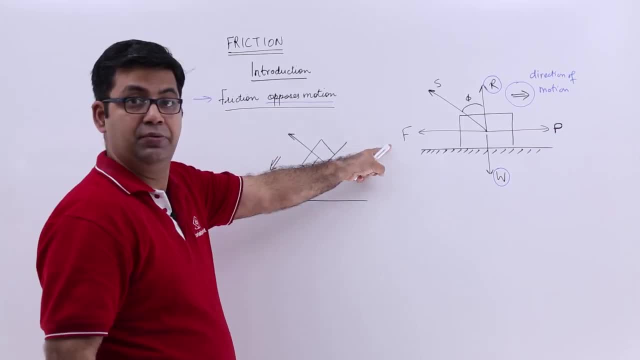 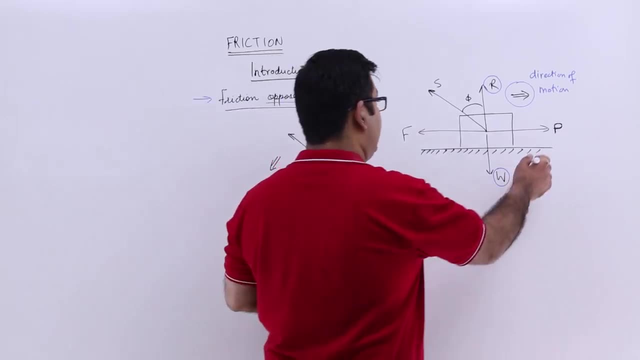 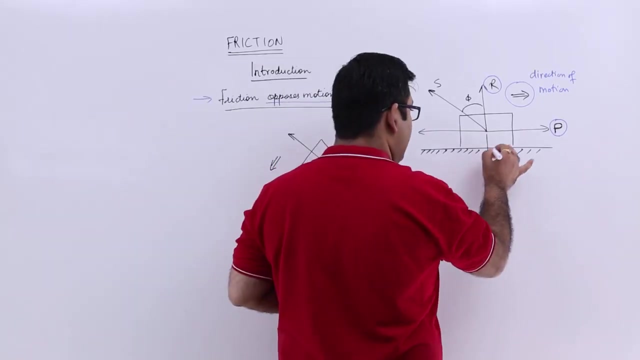 is the opposite direction to the motion. So this acts to oppose the motion. always Do not look at the direction of the force being applied. No, You might have a force which is being applied in a inclined direction, but the motion is in this direction. So this is. 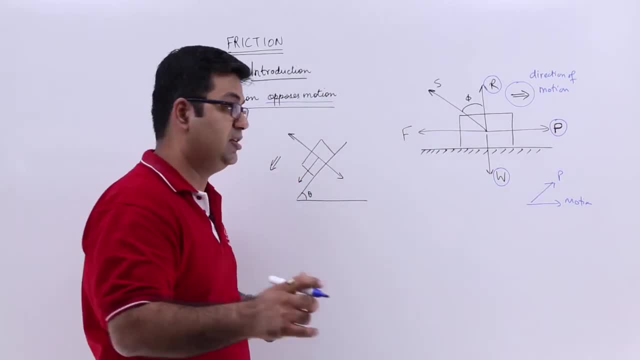 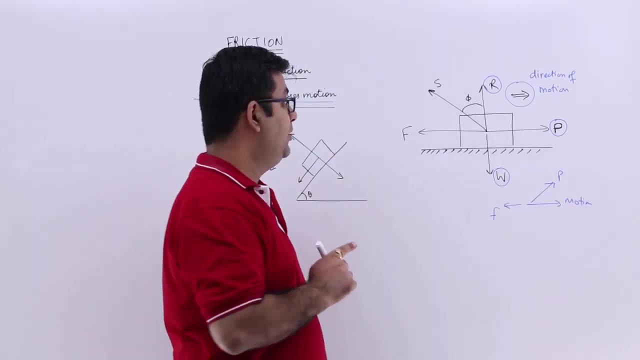 F aka F". Okay, so the force of friction will always be in the opposite direction to the motion, not to the applied force. Now, if you look at this frictional force and the normal reaction, let us give them names for the moment. So P here capital, P is the applied force, capital. 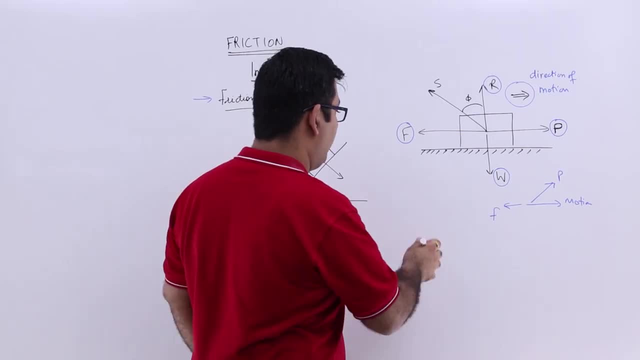 R: here this is normal reaction using normally flying or non- Athenian force. Now let me say here C, here capital A, here this is the applied force. capital P: here this is normal reaction using normal reaction. Now, if we look here, capital T: here this will been applied force. OK, Capital. 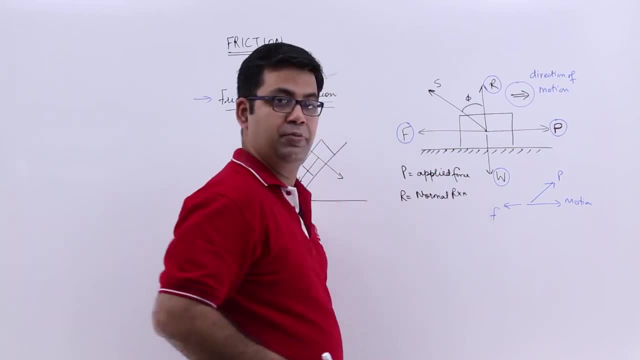 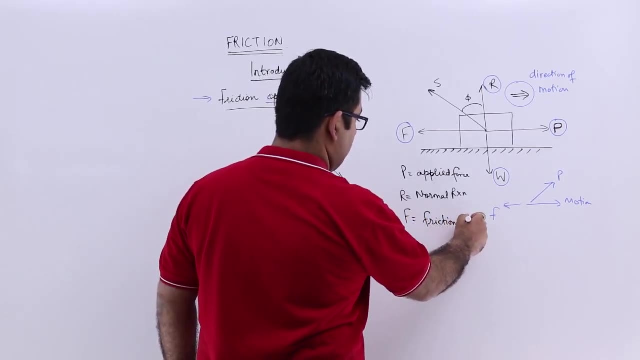 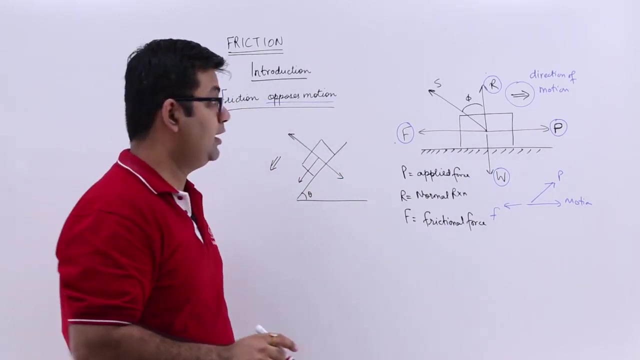 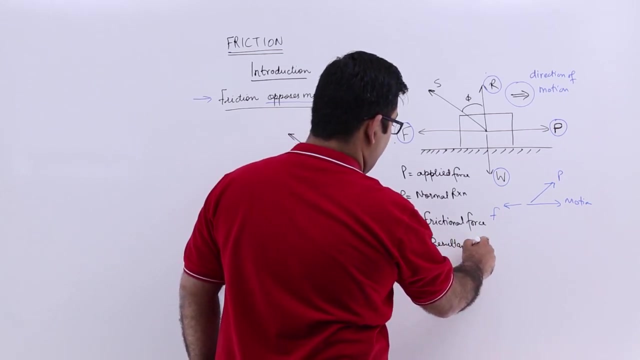 R here. this was the normal reaction in the circuitaptia, As you can see. so reaction: okay. then you have f, which is the frictional force. okay, now the resultant of f and r is s. so this is the resultant of friction and normal reaction. and if you look at this, 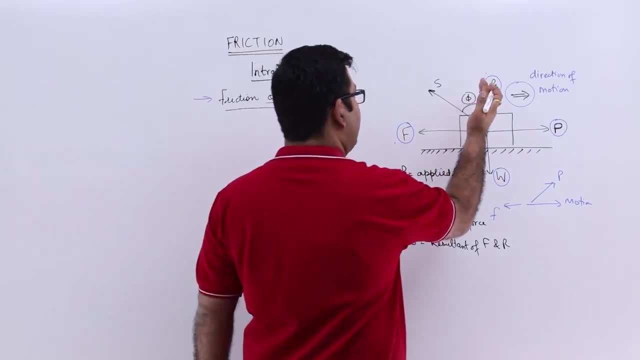 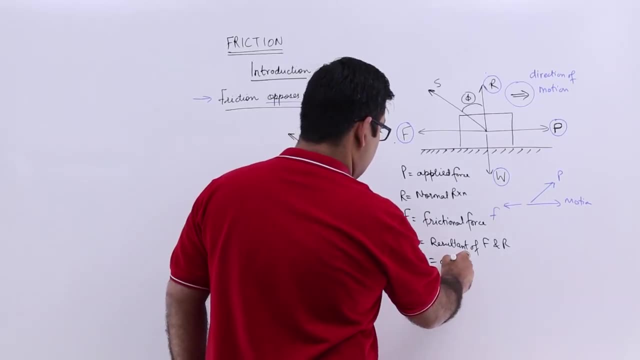 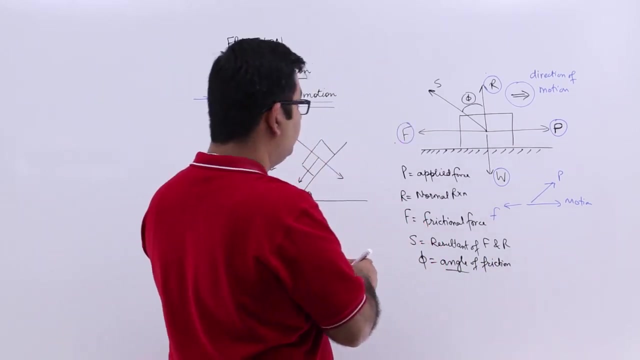 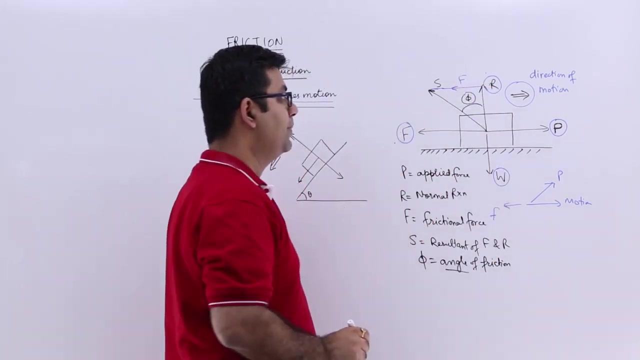 angle phi, which is the angle between the normal reaction and the resultant, between the friction and the normal reaction. this is called angle of friction, this is called angle of friction. so if i draw this f force over here, so this is f. and if i find out tan of this phi, tan. 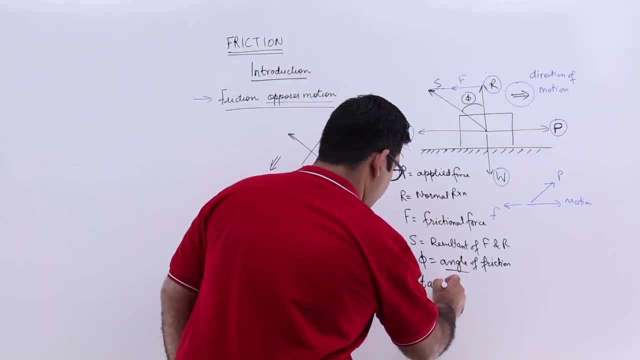 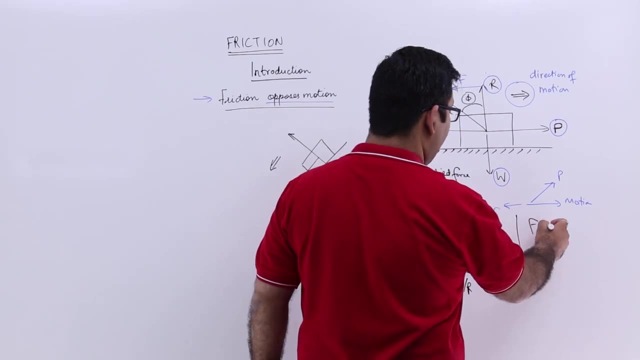 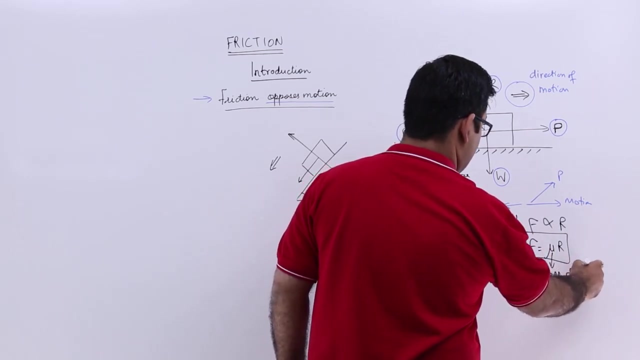 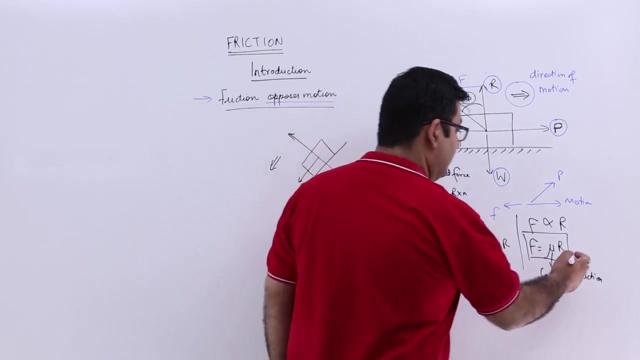 of phi is f upon r, and also we know that the frictional force is proportional to the normal reaction means f is equal to mu, r, where mu is the coefficient of friction. it is the coefficient of friction. so tan phi is f by r. now if you look at this expression, the value of f by r would be mu. so i can say that tan. 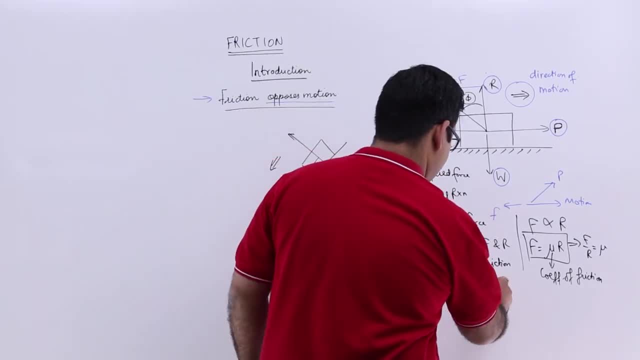 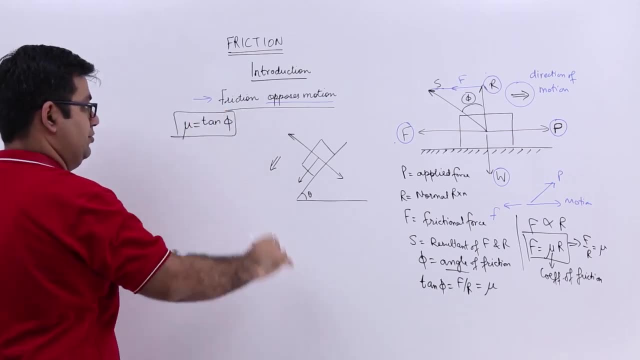 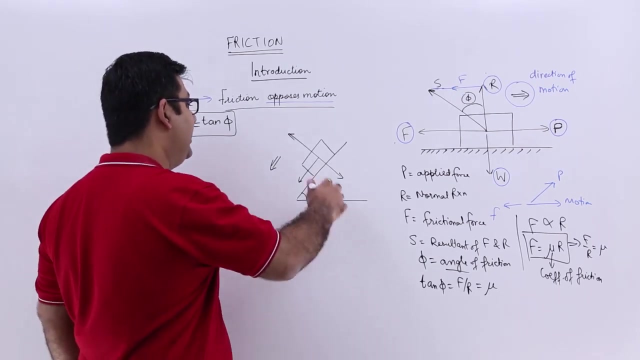 phi equal to f, by r equal to mu, so we can replace mu by tan of angle of friction. okay, similarly, we can analyze a block sliding downwards on an inclined plane which is at an angle of theta to the horizontal faceriction of my event value. there is an angle called regular. 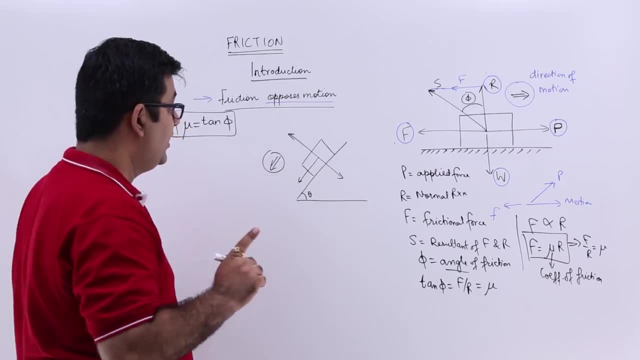 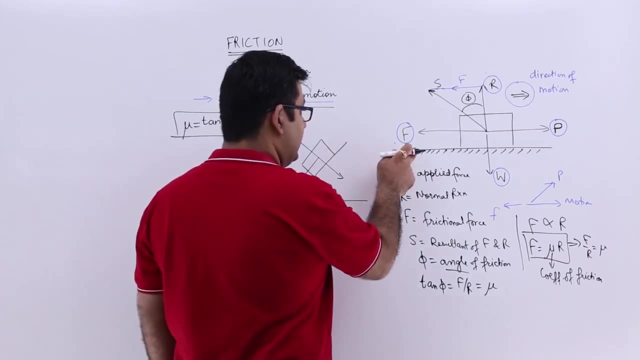 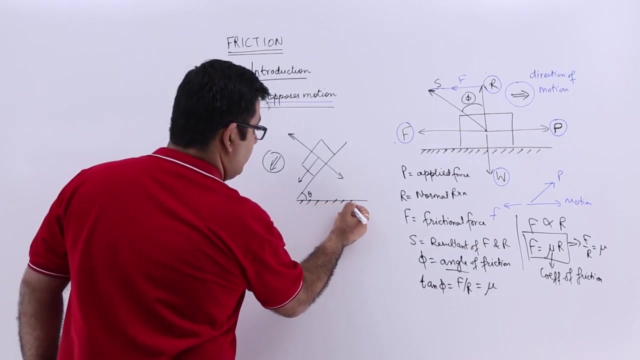 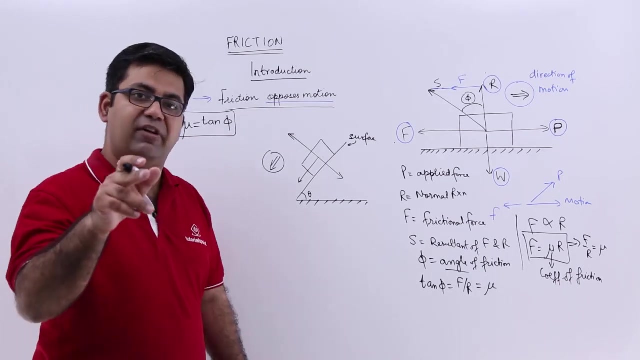 now remember one thing: weight of the body will always act normal to the ground. okay, so this is the. in this case, the ground and the surface are same, but over here, this is ground and this is surface, the inclined surface. okay, so your weight will always be acting. 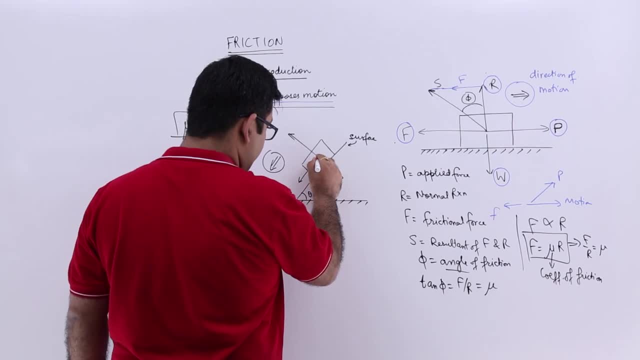 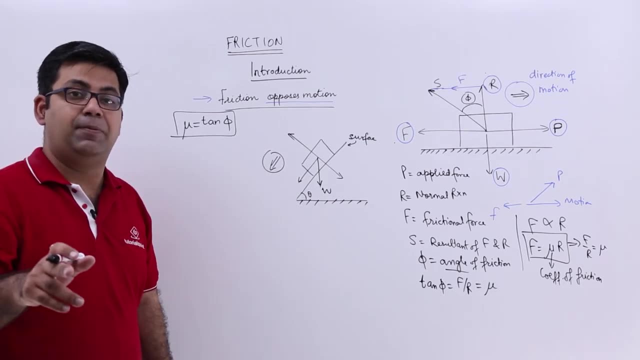 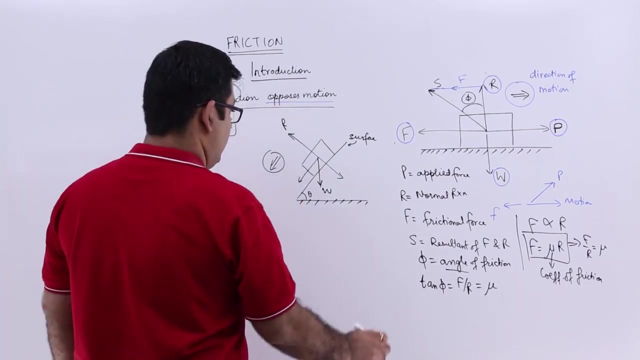 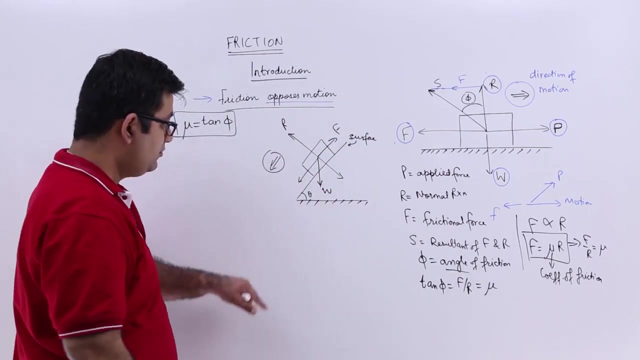 perpendicular to the ground. okay, so you will have, like this, weight acting perpendicular to ground and your normal reaction is always perpendicular to the surface. so this is r? okay, let us say this is the direction of motion. your friction would be this side. this angle is theta. then this will also be theta by geometry and this would be: 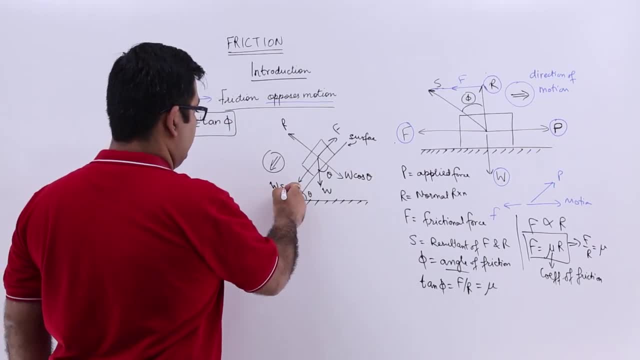 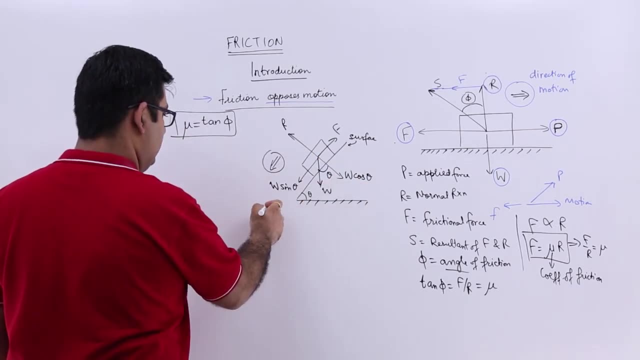 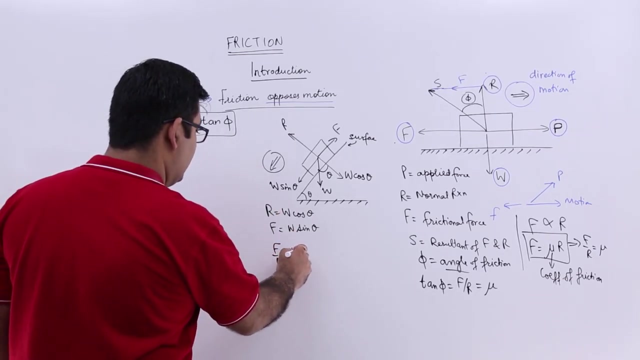 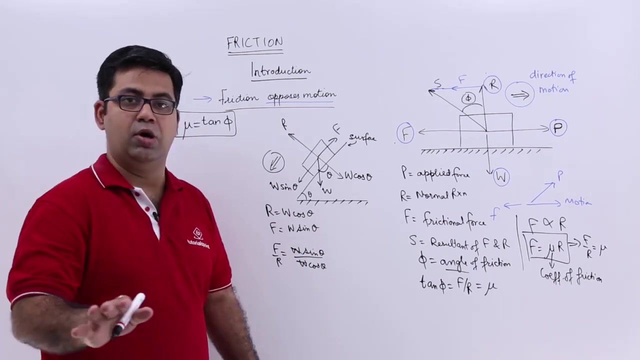 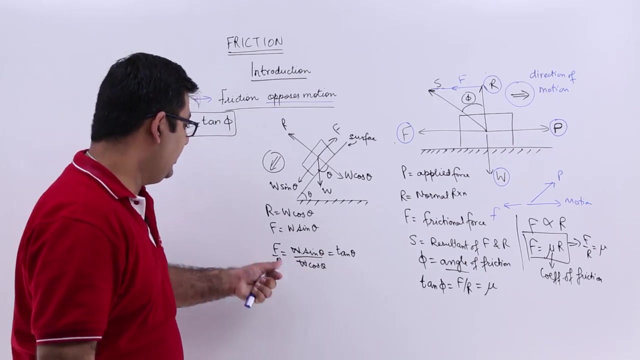 W cos theta, and this would be W sin theta. I can say that R is equal to W cos theta and F is equal to W sin theta. Let us divide them. You will have F by. R is equal to W sin theta upon W cos theta. W and W gone Sin by cos is tan So tan theta. Now, what is tan F by?